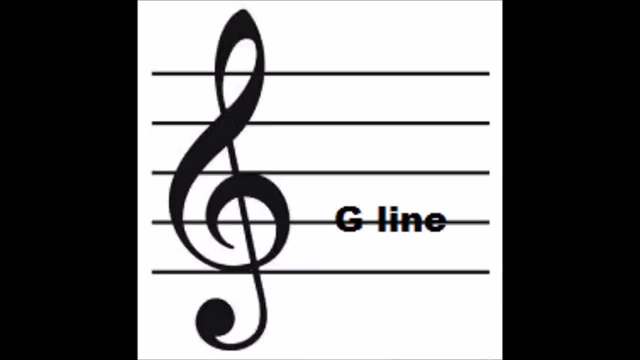 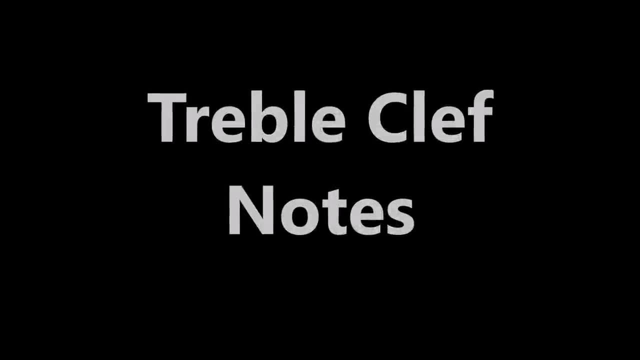 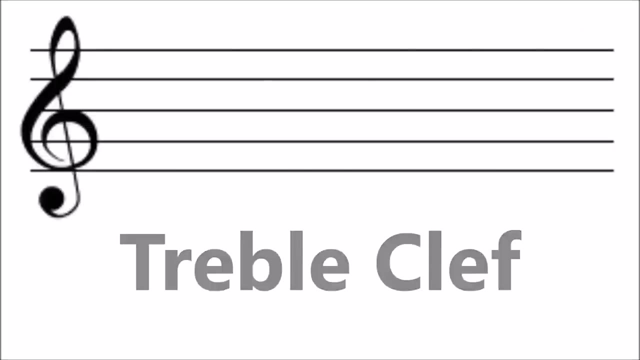 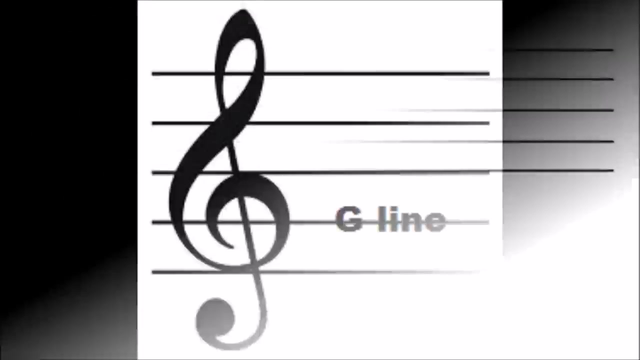 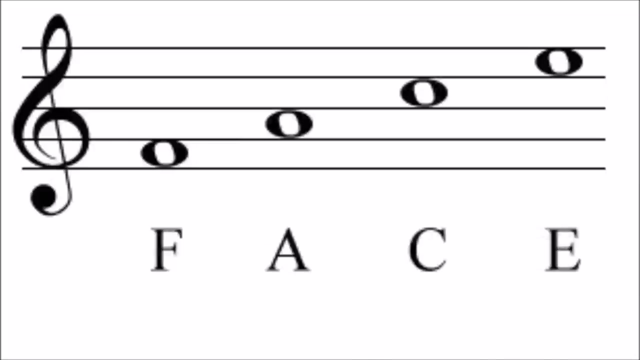 Here's a treble clef with G-line labeled Treble clef notes. Let's say we have a treble clef. This clef is also known as a G-clef because it wraps itself around the G-line Space notes F-a-c-e. 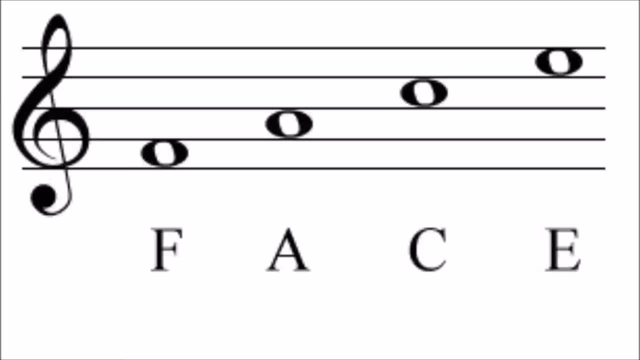 Let's have a look at the notes in the spaces. The notes in the spaces of the treble clef spell the word face, Starting from the bottom. the first space is named F. The second space is named F. The third space is named F. 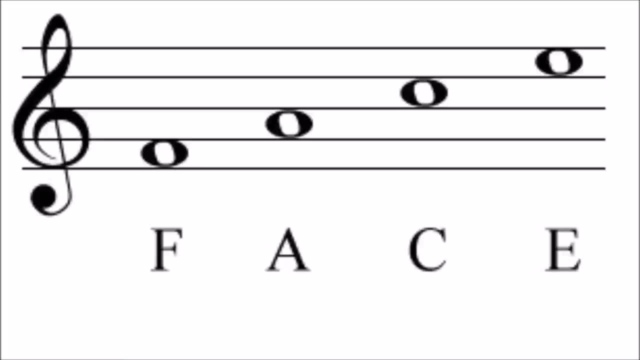 The fourth space is named F, The fifth space is named F, The sixth space is named F, The seventh space is named F? A, The third space is named C and the fourth space is named E, F, A, C, E. 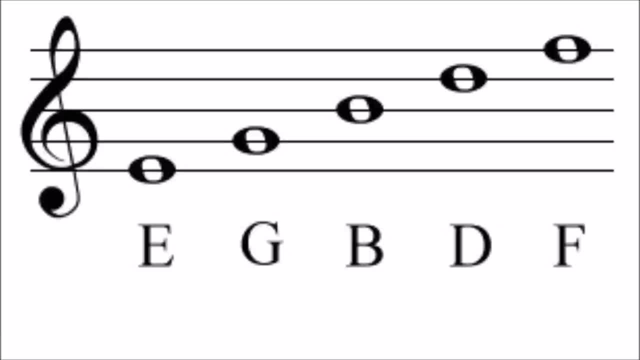 Line notes E, G, B, D, F. Notes on the line starting from the bottom are as follows: The first line is named E, The second line is named G, The third line is named B, The fourth line is named D. 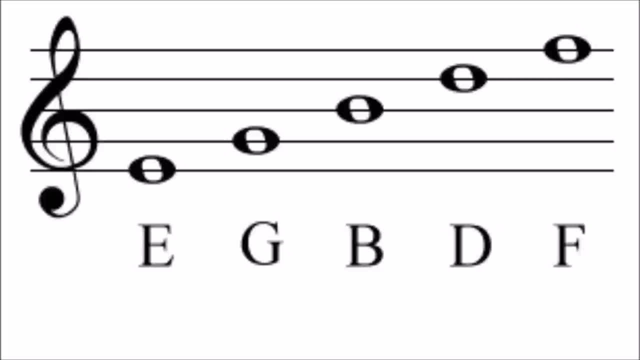 And the fifth line is named F. This results in E, G, B, D, F. Since these letters do not spell a word, you can use a phrase to help you remember the order. A common phrase is: every good boy deserves football. 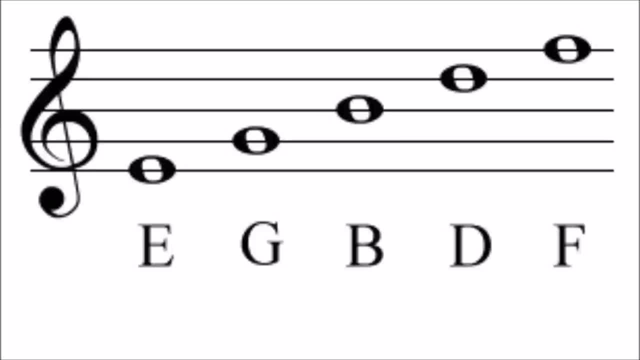 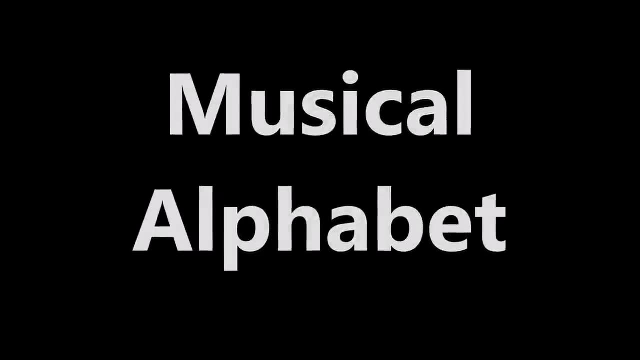 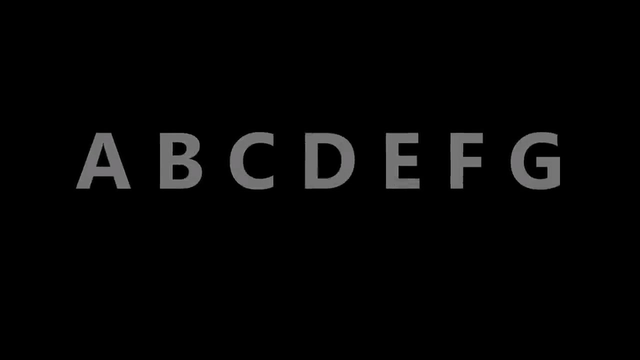 Or you can say: every green bus drives fast. It's all up to you. You can come up with your own phrase if you like. Notes are based on the first seven letters of the alphabet: A, B, C, D, E, F and G. 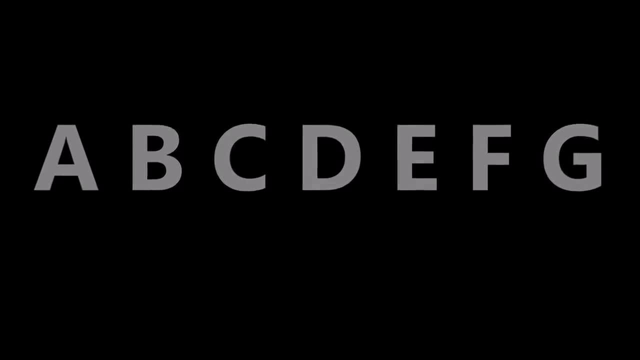 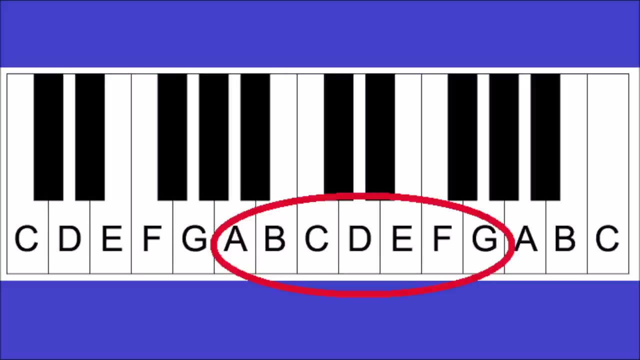 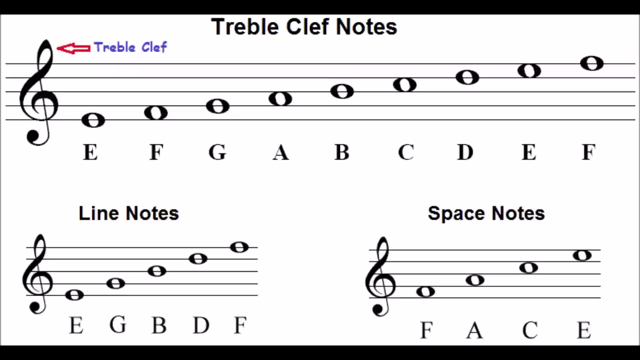 This is known as the musical alphabet. When you get to G, you go back to the beginning of the alphabet. In other words, after G you go back to A and not H. If we take all the notes of the lines and spaces of the treble clef and place them on the staff. 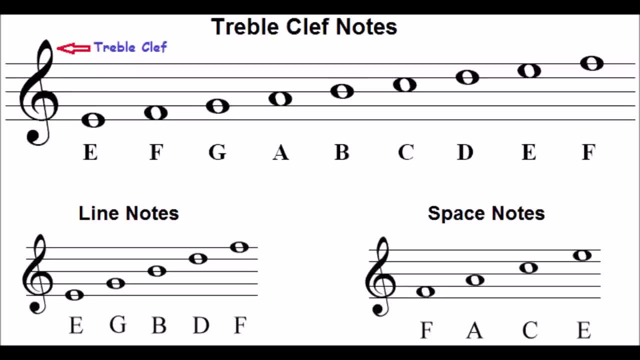 we will notice that the notes simply move in alphabetical order. Treble clef notes: E, F, G, A, B, C, D, E, F. Line notes: E, G, B, D, F. Space notes. 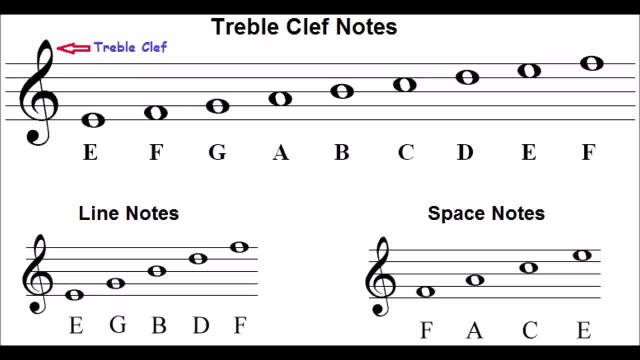 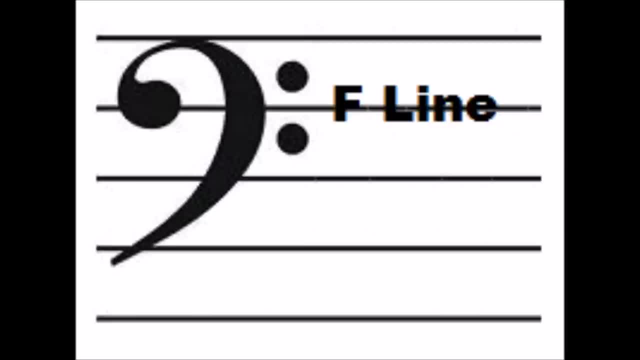 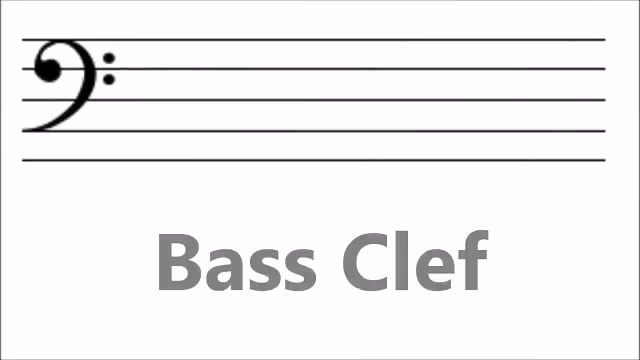 F, A, C, E. Here's a bass clef with F line labeled Bass clef notes. Let's now take a look at the bass clef. This clef is also called the F clef Because historically. 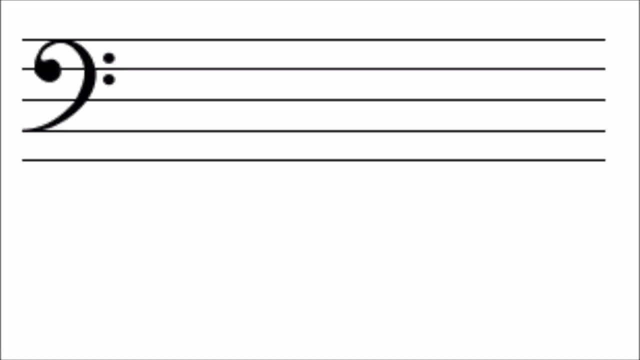 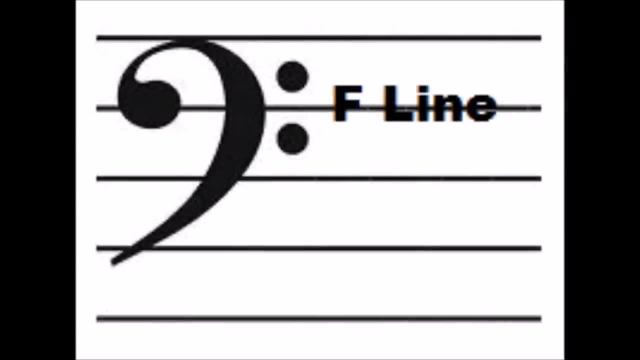 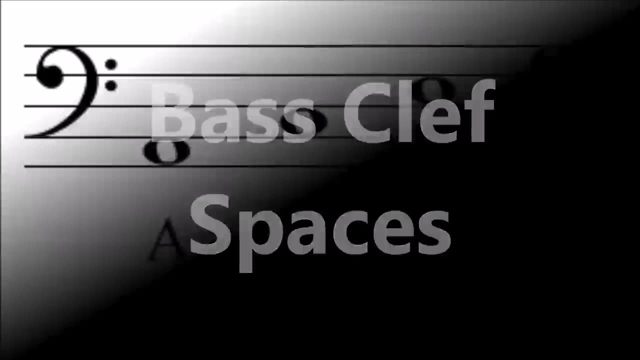 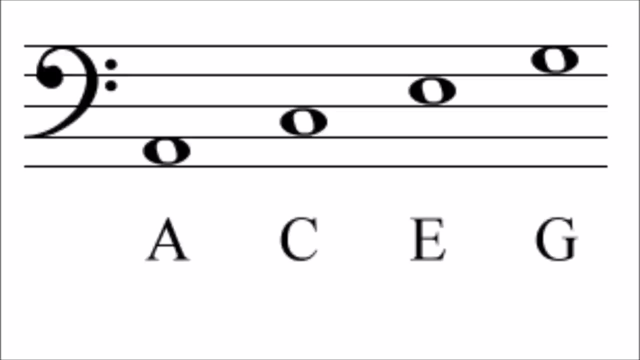 it looked like the letter F. Also, the two dots of the bass clef sit on either side of the F line. Bass clef spaces A, C, E, G. The names of the notes on the spaces of the bass clef are as follows. 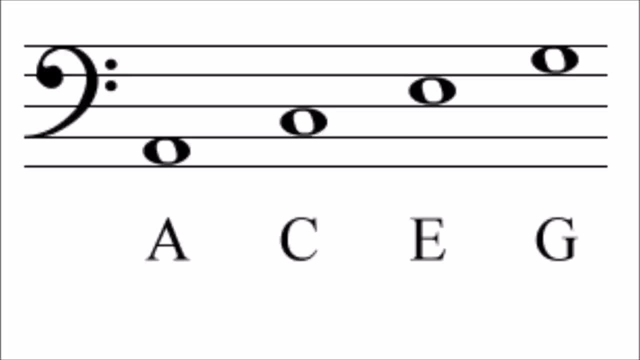 of the bass clef as follows: the first piece from the bottom is named a, the second space is named C, the third space is named E and the fourth piece is named G. this results in a, C, E, G. a common phrase used by musicians to remember these notes is all cows eat grass. another phrase is all cars eat gas again. 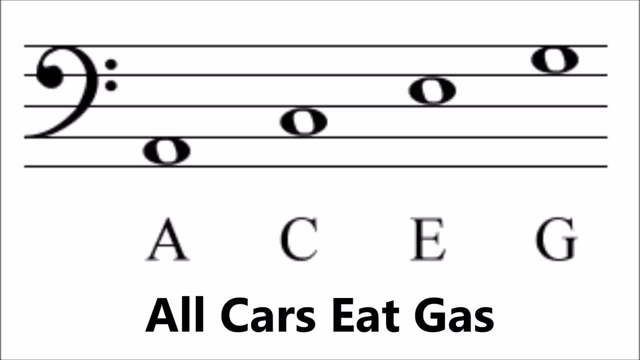 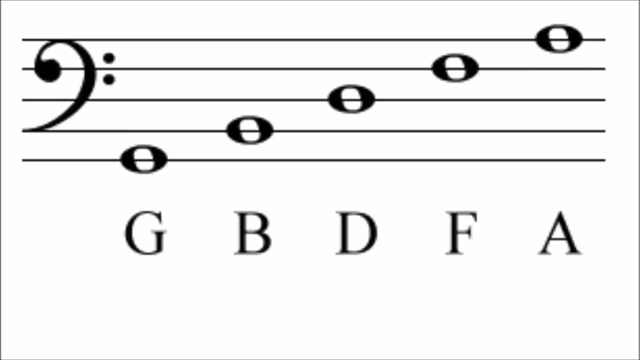 you are free to come up with a new phrase like this one, with any phrase you like, as long as it helps you remember the names of the notes. bass clef lines G, B, D, F, E, the notes of the five lines of the bass clef as follows: line one is named G. 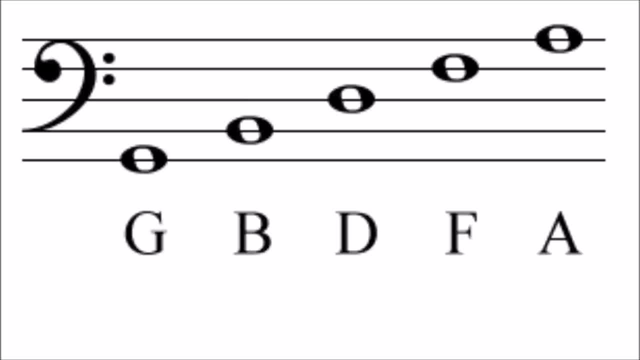 line two is named B, line three is named D, line four is named F and line five is named a. this gives us G, B, D, F, E. there are quite a few phrases that we can use to compare all the five. they sound like a set of cursive. IFлемM and Woulda have a. 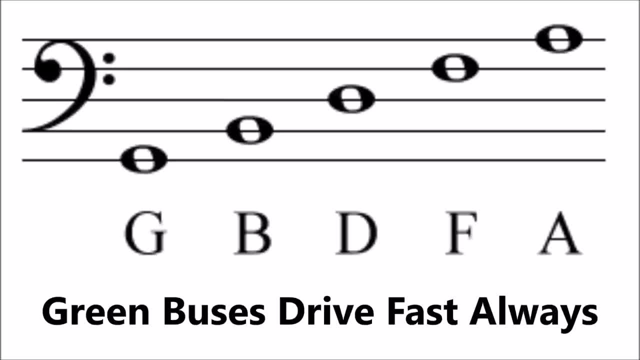 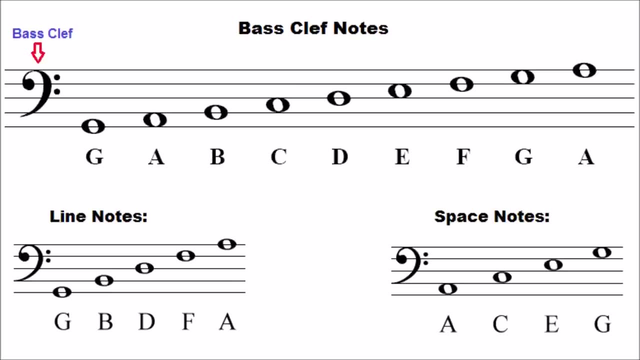 there are quite a few phrases for this, such as green buses drive fast always, or good boys deserve football always. if we take all the notes of the lines and spaces of the bass clef and place them on the staff, we will notice that the notes on the bass clef notes aren't just numbers. they are here and there. and places of the bass clef and they are all forms of bonds and, uh, you will notice, all these is an order or text and fractions on the top and bottom of certain. you don't need to write and the stretch them, just numbers as becuase your orientation is exactly what we did this time, for. 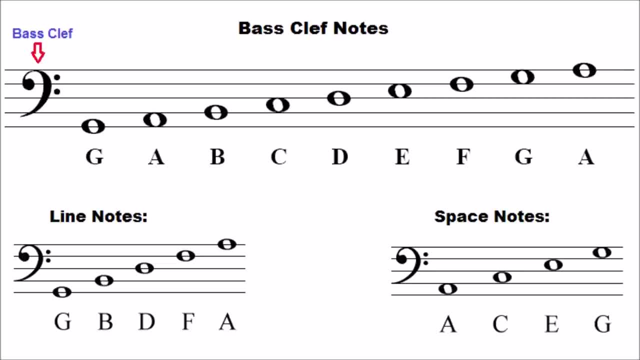 The notes simply move in alphabetical order. After G you go back to the first letter of the alphabet, which is A, then B, C, D, and so on. Base clef notes: G A, B, C, D, E, F, G, A. 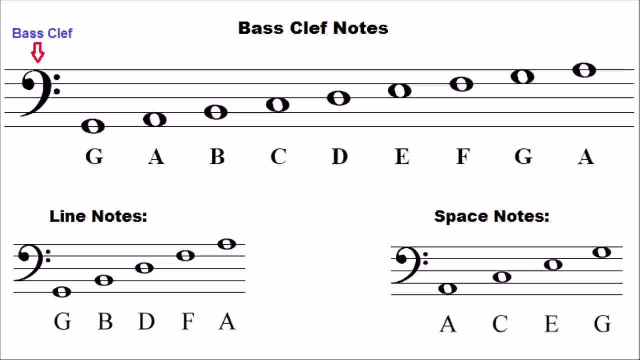 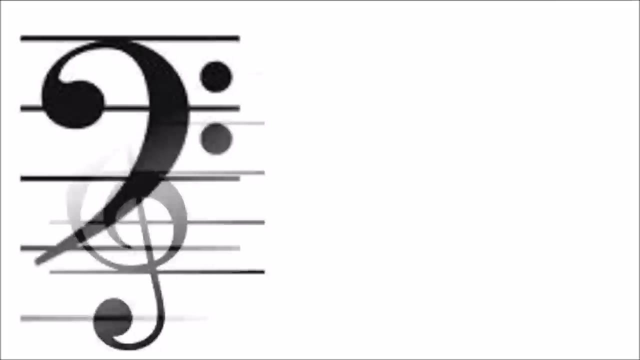 Line notes of the base clef: G, B, D, F, A. Space notes A, B, C, D, E, F, G, A, C, E, G. Practice drawing: treble clefs and bass clefs. 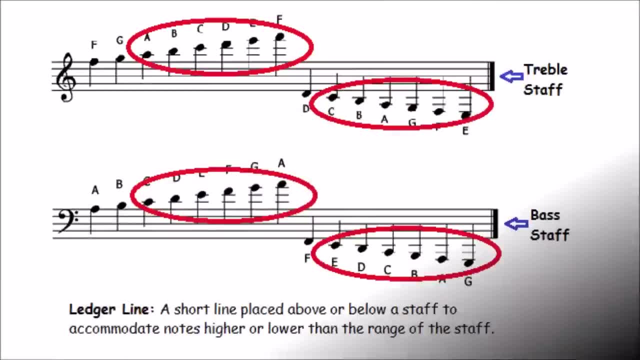 Ledger lines. Let's say we want to play higher or lower notes than what the bass and treble staff cater for. How will we achieve that? Where will we replace these notes? After all, there are many more notes on a musical instrument than the few notes we looked. 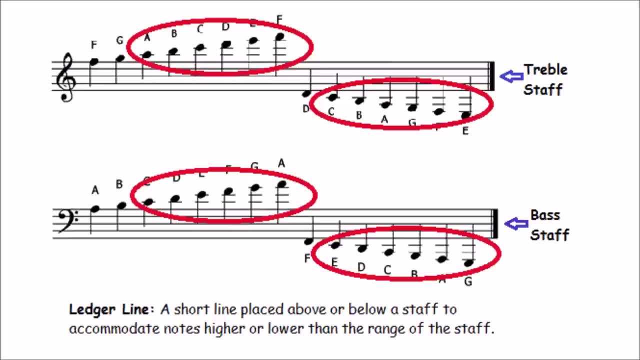 at earlier. To accomplish this, ledger lines are used L-E-D-G-E-R lines also spelled L-E-G-E-R. L-E-G-E-R are short lines placed above and below the staff. They are used to help us extend beyond the range of the staff. 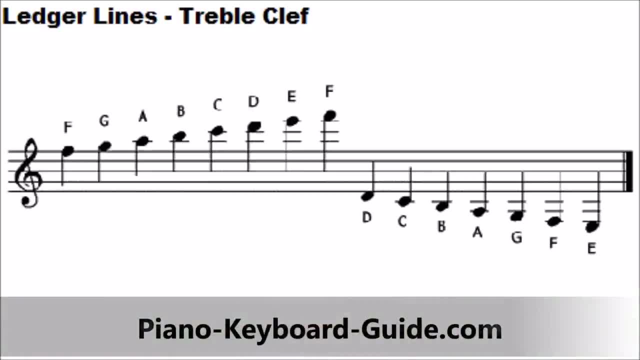 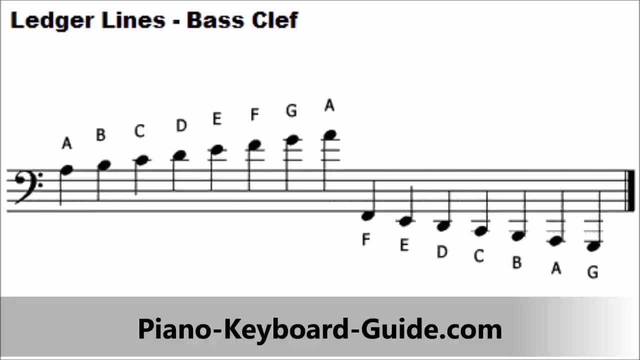 Ledger, lines A, B, C, D, E, F, C, B, A, G, F, E, C, D, E, F, G, A, E, D, C, B, E, C, D E, F, G A G. 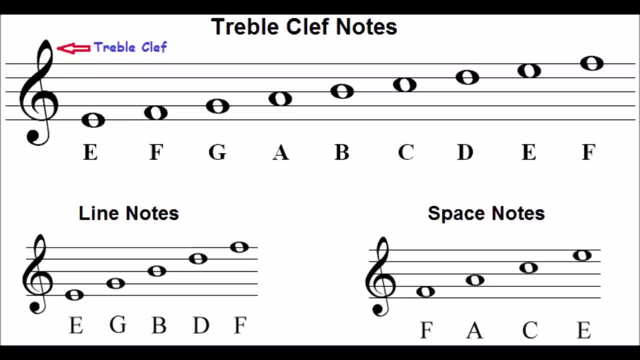 Let's take the treble clef, for example. As we saw earlier, the notes on the lines of this clef are E, G, B, D, F And the notes of its spaces are F, A, C, E. 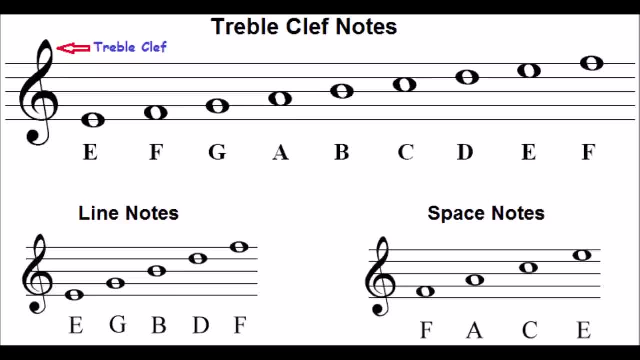 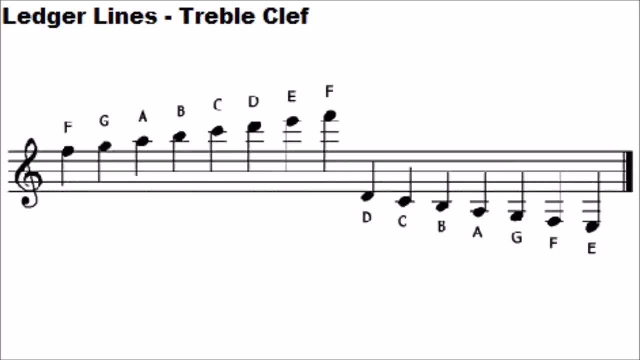 When we combine these notes we get E, F, G, A, B, C, D, E F. The note after the 5th line of the treble clef is G. To add the note after G, which is A: 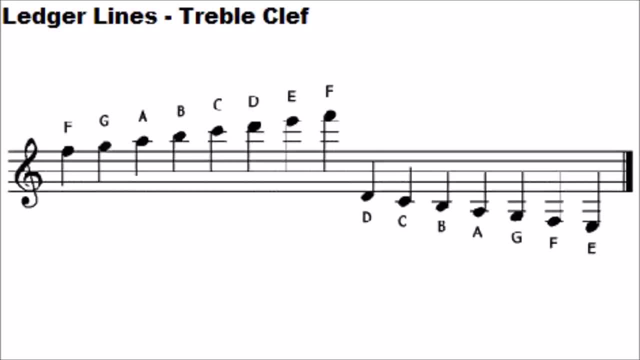 we need a ledger line. The first ledger line is A, The note after A is B. We need another ledger line to add the note after B. So the second ledger line is C, The third ledger line is E. These three ledger lines. 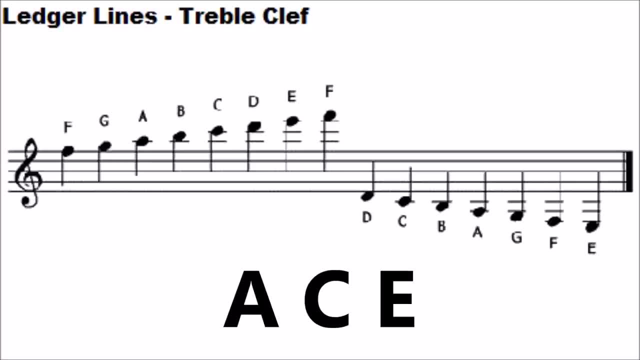 spell the word ace. That's A, C, E. This makes it easy to remember. Notes can keep going higher and higher on the treble staff by simply moving in alphabetical order. Notes go lower as well, as can be seen in the alphabetical order. 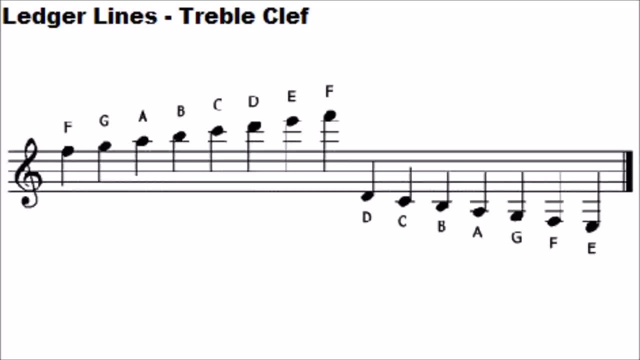 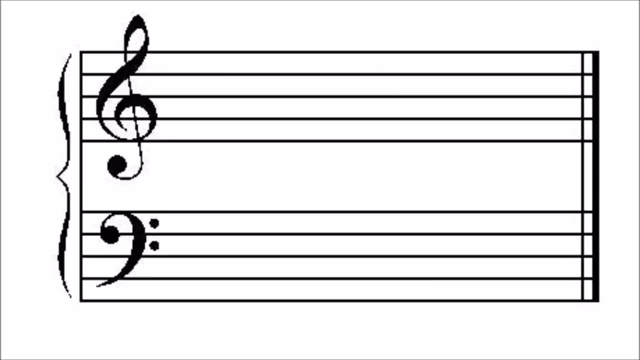 The first one is three, the second one is four. This makes it easy to remember. Notes go lower as well, as can be seen in the alphabetical order, Notes go higher and in the ledger lines diagram, The treble and bass clefs are often combined to create. 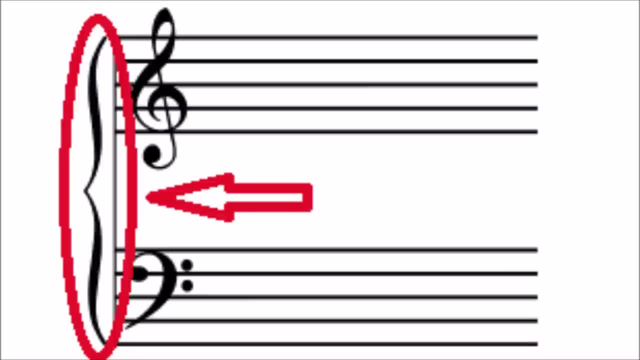 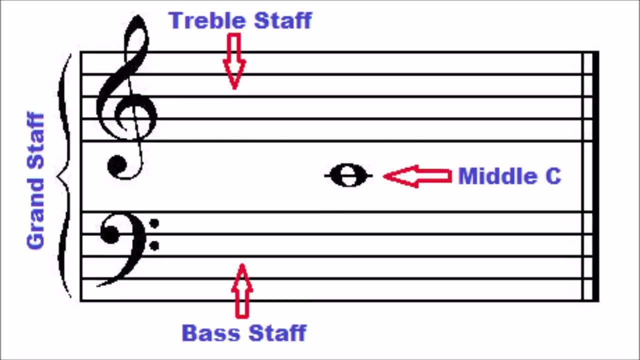 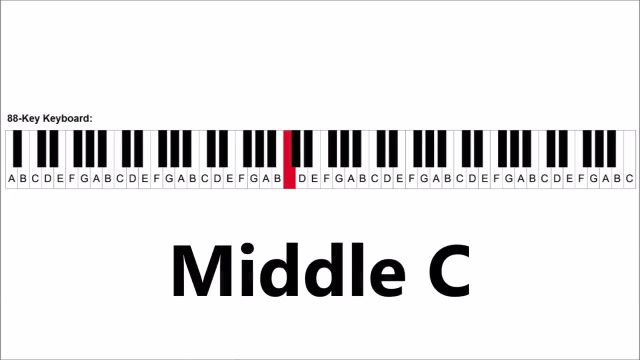 a grand staff A perpendicular line and bracket, called a brace, is used to join the two staves together. The note in the center of the grand staff on a ledger line is middle C. On piano, middle C is the centermost C. It is near the middle of the keyboard. 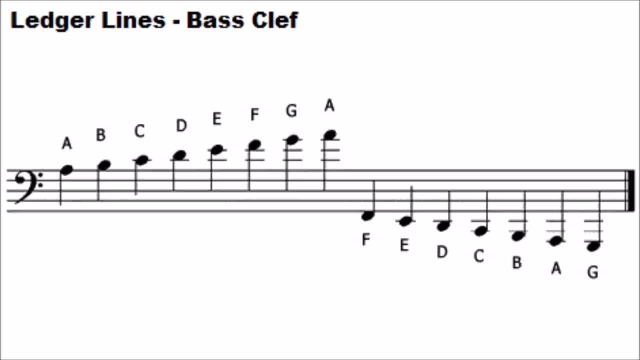 The three ledger lines below the bass clef are the middle C. The three ledger lines below the bass clef are the middle C. The three ledger lines below the bass clef are the middle C. Spell the word ace as well, in ascending order. 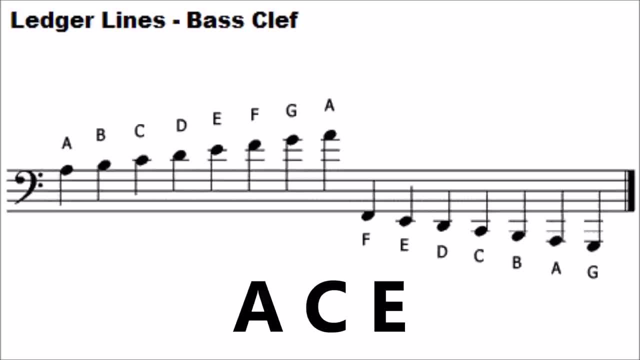 That's A, C, E. We can keep adding ledger lines below the note A. for notes which are much lower, Ledger lines can be placed above the bass clef as well. The notes seem to simply move in alphabetical order. The note of the fifth line of the bass clef is A. 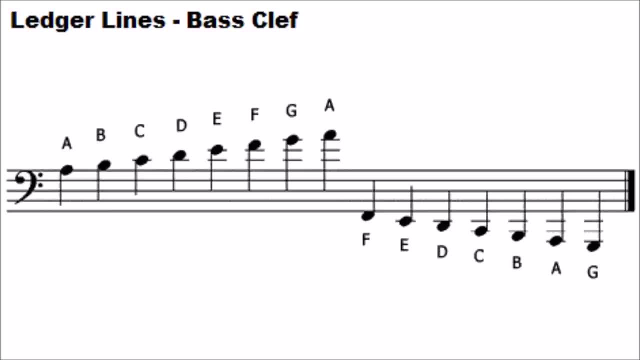 The note after A is B, Then C or middle C. Middle C, as we've seen, is on a ledger line. The note after middle C is D. D must be placed above this first ledger line, But if we need to add the note after D, which is E, we would need another ledger line. 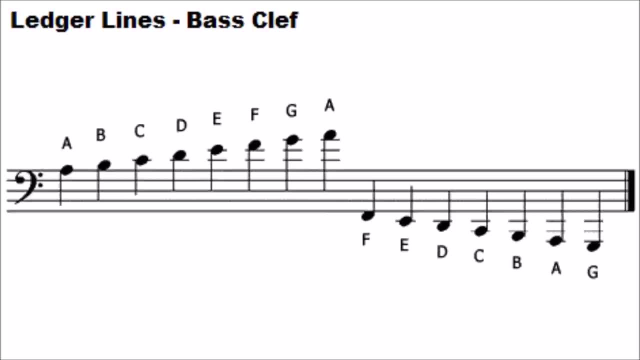 This would give us two ledger lines. Then the note after E is F. The note G would not be placed above this first ledger line. Now we placed on yet another ledger line, giving us a total of three ledger lines. The more ledger lines that are added, the more challenging the music gets. 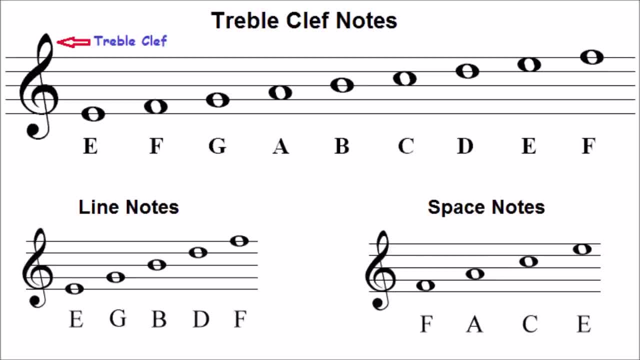 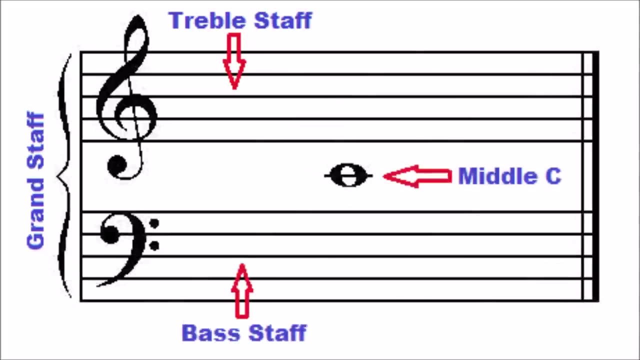 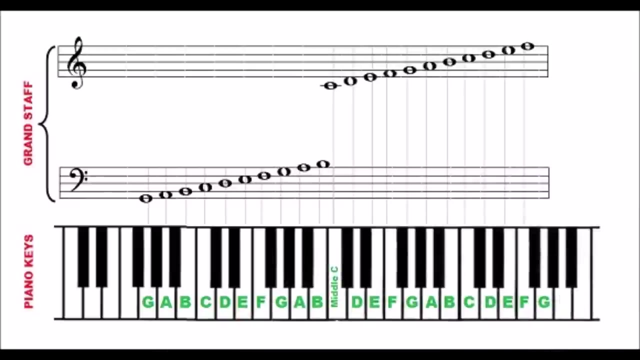 Therefore, for now, I want you to focus mostly on the lines and spaces of the treble and bass clef, As well as middle C. It all happens one step at a time. Note on the staff and how they correspond to piano keys. That's enough for today. Let's get back the music To learn the F I as before. please remember the same thing as A before and after. We stumbled over the other two mac and finished the A before and after, And therefore we now understand the scale at which the notes stop, but are the opposite. Repeat Note C, B, G, F, D, F, G.